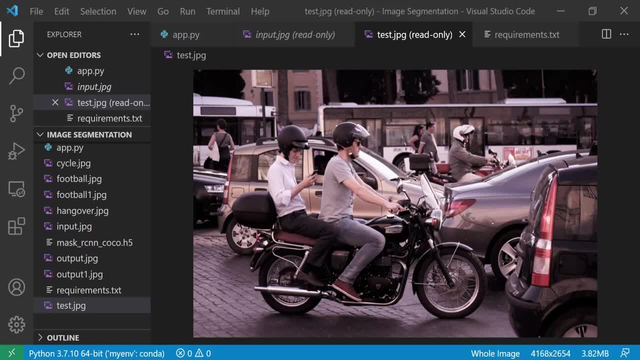 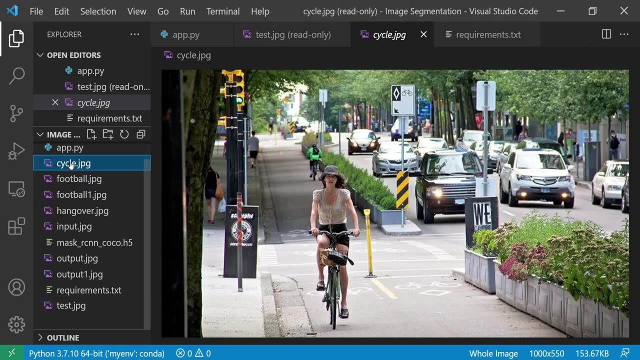 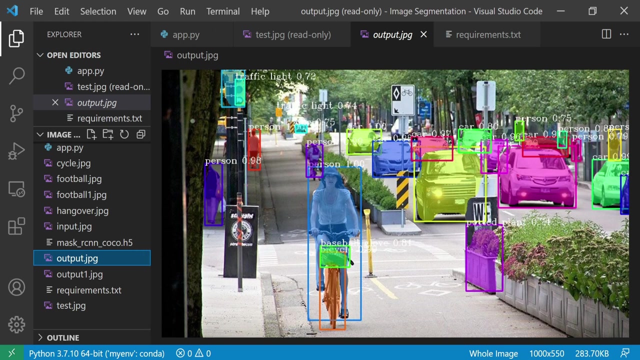 Hello, all my name is Krishnak and welcome to my YouTube channel. So, guys, this will be an amazing video for every one of you, because in this particular video, we are going to discuss about image segmentation and how you can implement it with just writing five lines of code, right? So initially, if you have this kind of image- or probably you have this kind of image- then you will be able to convert it something like this: Okay, now, here you can see that how the segmentation is basically done. So object detection is also there. You can see over here traffic light, person, everything. 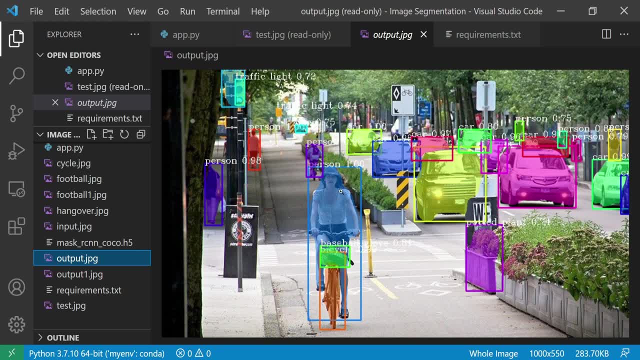 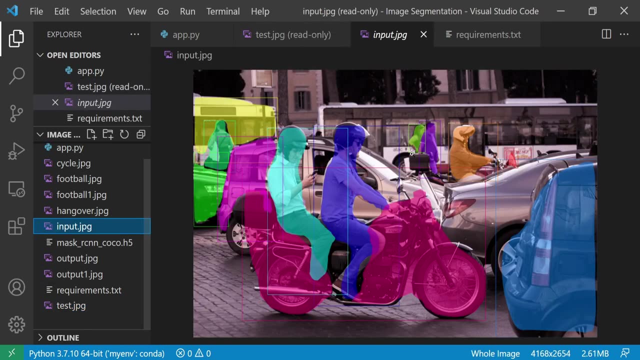 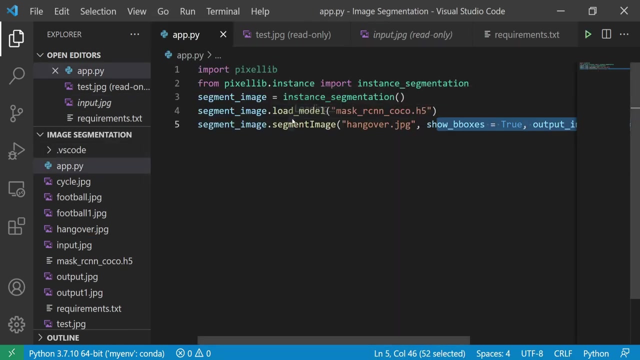 is there? Apart from that, the segmentation you know it is being able to do this kind of segmentation where, with different, different colors, you'll be able to see each and every objects, and into this right, Not only this. suppose, if I have this specific image, if I apply this kind of segmentation, then finally you'll be able to get something like this right, And this is all possible just by this five lines of code, right? So we'll try to see what it is, And the library that we are going to use is pixel lib. So what is pixel lib? over here you can see. 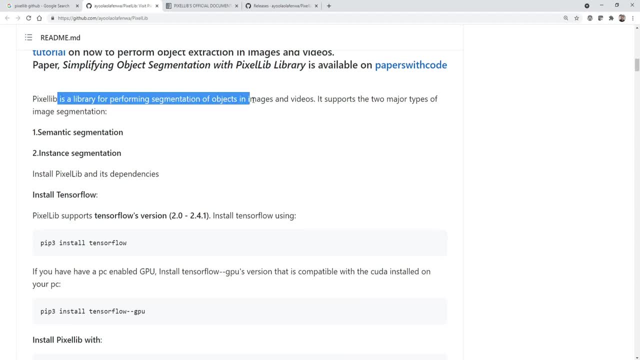 the pixel lib is a library for performing segmentation of objects in images and videos, So it both supports, both in images and videos. Right now, in this particular video, we'll focus on images, you know, and then in the upcoming videos we'll see in videos how we can do it right. It'll be pretty much amazing. I tried it with both And, trust me, with the approach that we used to follow before and with the approach of this, you'll be able to do it very, very easily. And here you can also do custom training, which I will be showing you as we go ahead. Okay so, 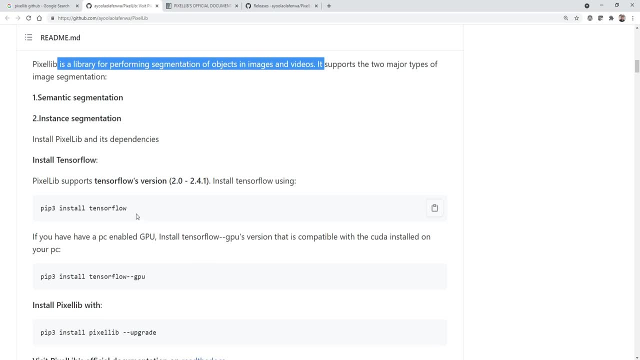 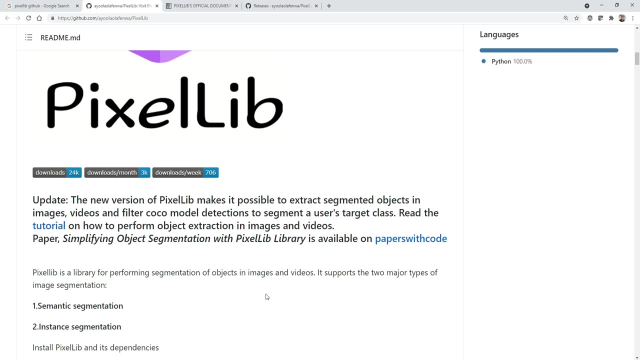 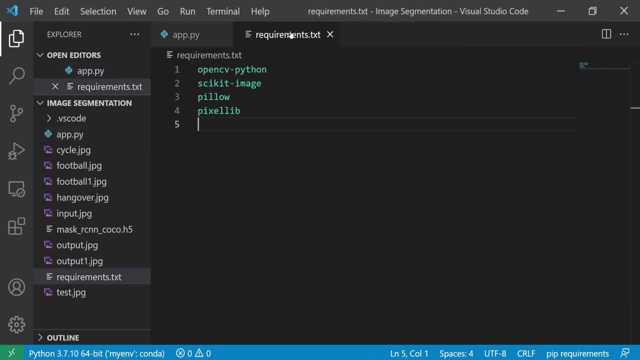 for this. first thing is that: what are libraries you actually require? you require TensorFlow, you require TensorFlow GPU- any of them- And there is also some dependencies of libraries that are required. Okay, And you can also check out this entire GitHub page. So let's proceed And let's see. First of all, I'm just going to create my requirementtxt file. So here you can see. these are my requirementtxt files which you actually require. Okay, One is OpenCV, Python, SkyKit image pillow pixel lib. Okay, so this: all libraries are required. 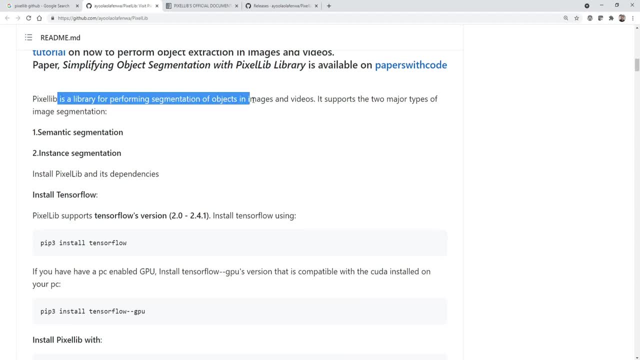 the pixel lib is a library for performing segmentation of objects in images and videos, So it both supports, both in images and videos. Right now, in this particular video, we'll focus on images, you know, and then in the upcoming videos we'll see in videos how we can do it right. It'll be pretty much amazing. I tried it with both And, trust me, with the approach that we used to follow before and with the approach of this, you'll be able to do it very, very easily. And here you can also do custom training, which I will be showing you as we go ahead. Okay so, 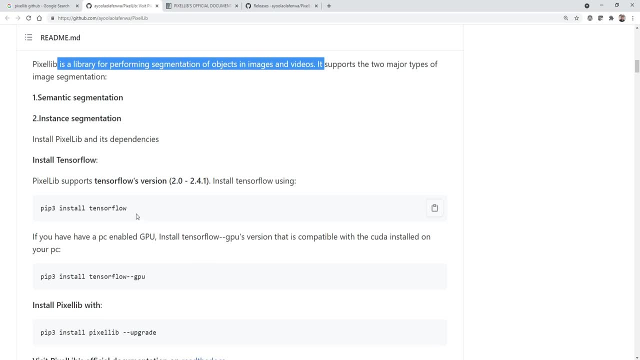 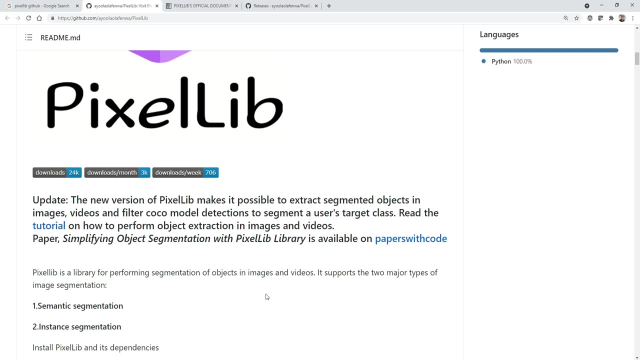 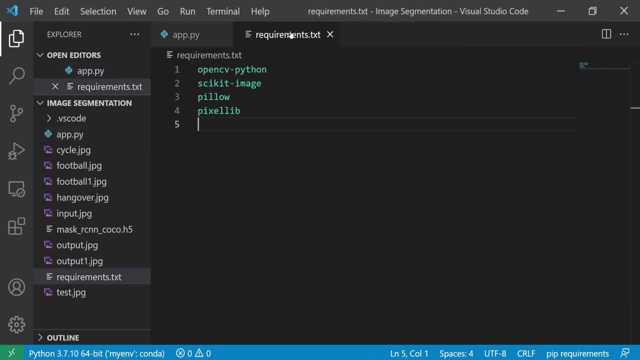 for this. first thing is that: what are libraries you actually require? you require TensorFlow, you require TensorFlow GPU- any of them- And there is also some dependencies of libraries that are required. Okay, And you can also check out this entire GitHub page. So let's proceed And let's see. First of all, I'm just going to create my requirementtxt file. So here you can see. these are my requirementtxt files which you actually require. Okay, One is OpenCV, Python, SkyKit image pillow pixel lib. Okay, so this: all libraries are required. 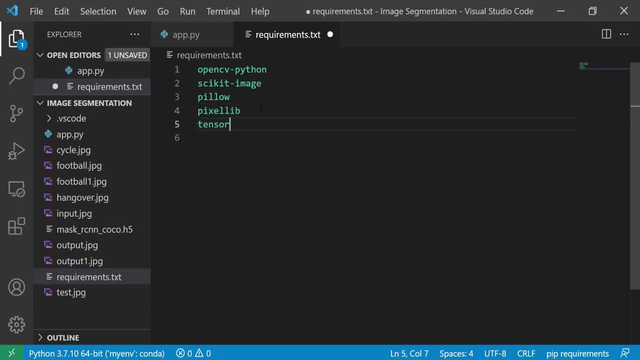 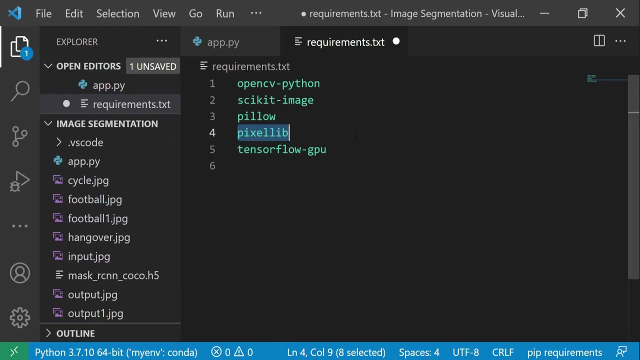 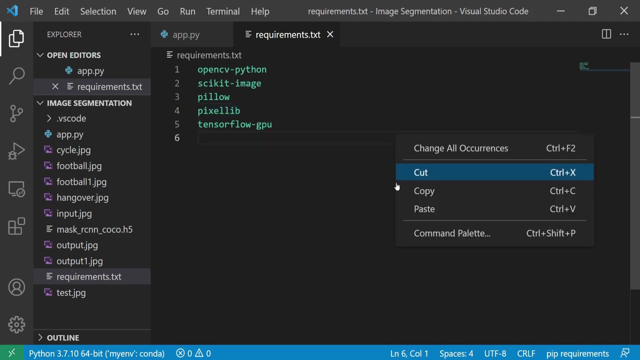 And one more which I forgot to write over here, is TensorFlow GPU, right? So this all libraries you actually require And this is the dependencies for this pixel lib library. Okay, at the end of the day, we are going to use pixel lib because there are techniques over here which will actually help you to do the image segmentation, both in images and videos, right? So please make sure that you keep this requirementtxt file and then go to the terminal and just write pip install. pip install minus. 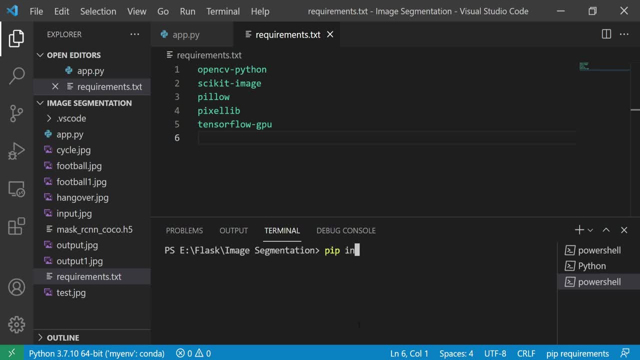 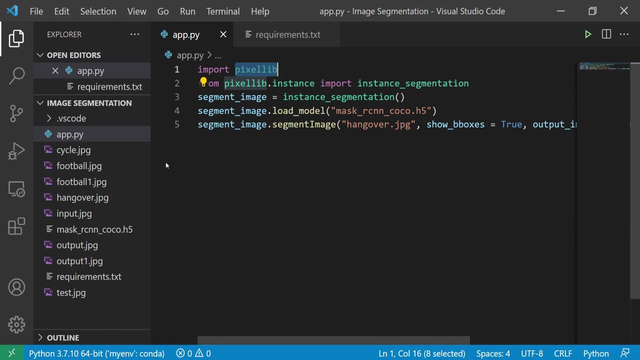 our requirementtxt. So you just have to write like this: pip install minus our requirement requirementstxt. That's it right? So automatically, all the requirements will be installed. Okay, I don't want to do it again because I have already done it. Okay, So let's go to the next step Now. the next step is that I will go to my apppy And in this particular code, what we are actually going to do is that we're going to import the pixel lab. we are going to import pixel labinstance import. 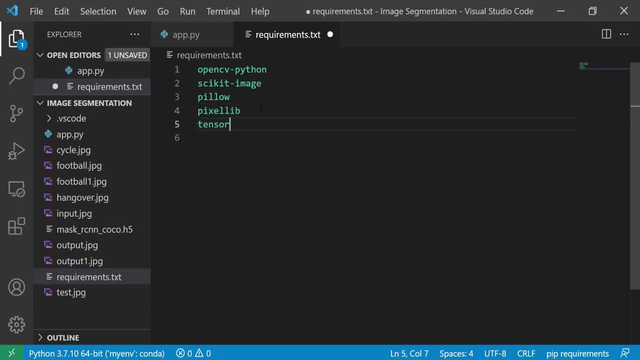 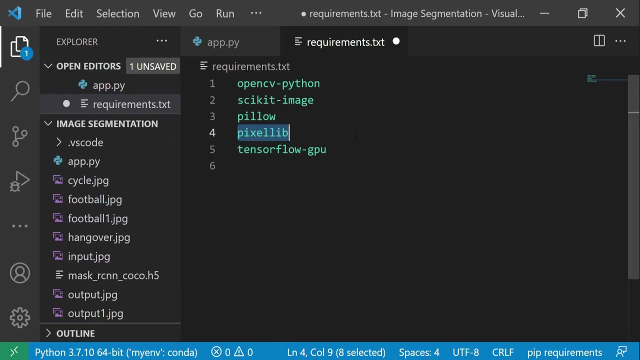 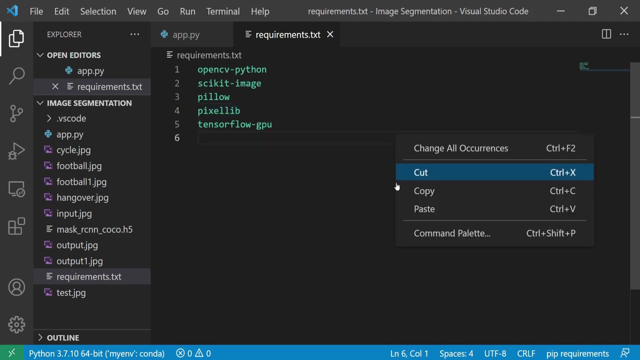 And one more which I forgot to write over here, is TensorFlow GPU, right? So this all libraries you actually require And this is the dependencies for this pixel lib library. Okay, at the end of the day, we are going to use pixel lib because there are techniques over here which will actually help you to do the image segmentation, both in images and videos, right? So please make sure that you keep this requirementtxt file and then go to the terminal and just write pip install. pip install minus. 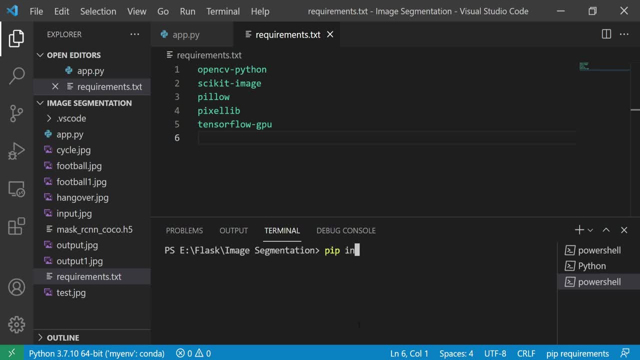 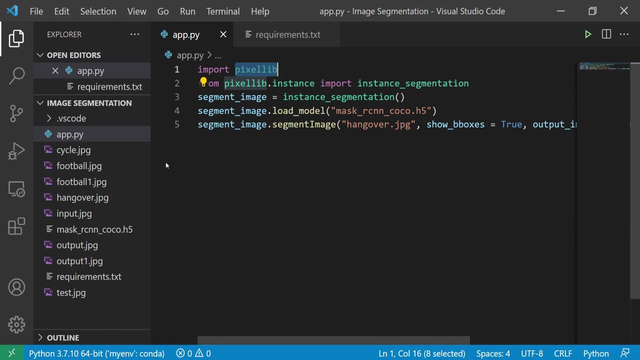 our requirementtxt. So you just have to write like this: pip install minus our requirement requirementstxt. That's it right? So automatically, all the requirements will be installed. Okay, I don't want to do it again because I have already done it. Okay, So let's go to the next step Now. the next step is that I will go to my apppy And in this particular code, what we are actually going to do is that we're going to import the pixel lab. we are going to import pixel labinstance import. 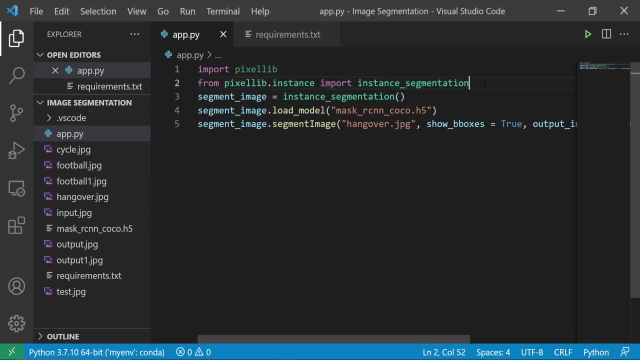 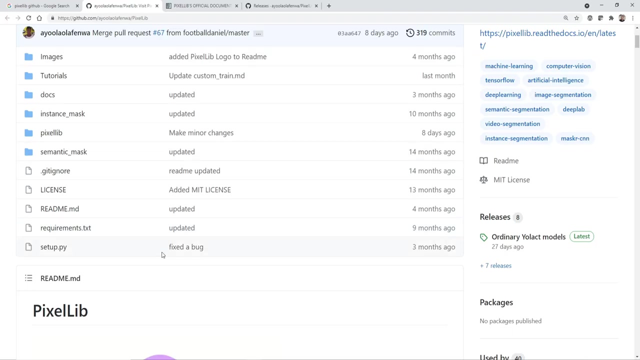 instance segmentation. So fine, guys, we have actually imported both this library and we are going to use this instance segmentation for doing the segmentation, And for this we also required a library, probably like our CNN, and also that it will be able to do the object detection And, based on that, it will also be able to show the boxes to us, right? So for that we are going to use this h5 file. And where did I get this h55?? Because it is already given away. if I go down, you'll be able to see all the examples over here, And they have released. 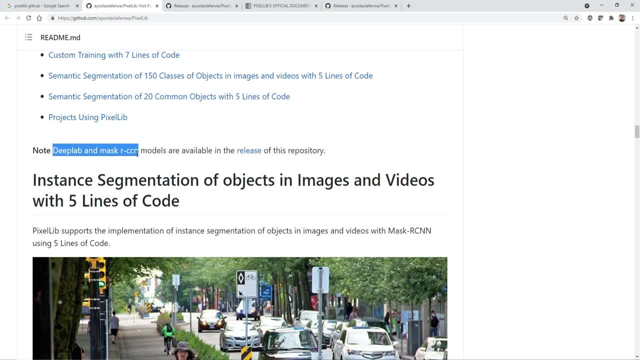 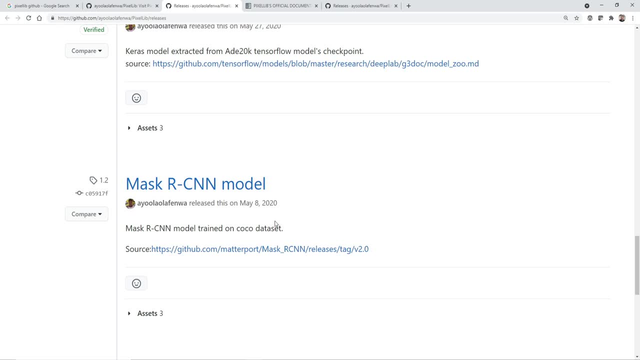 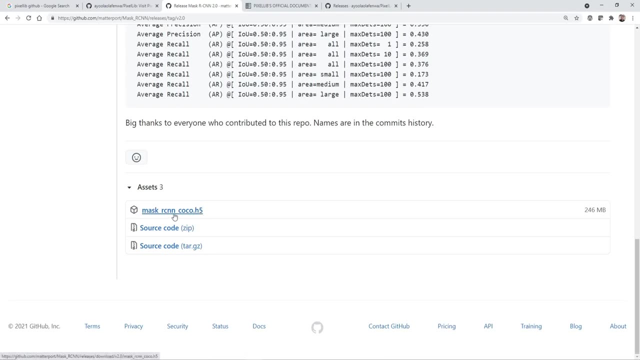 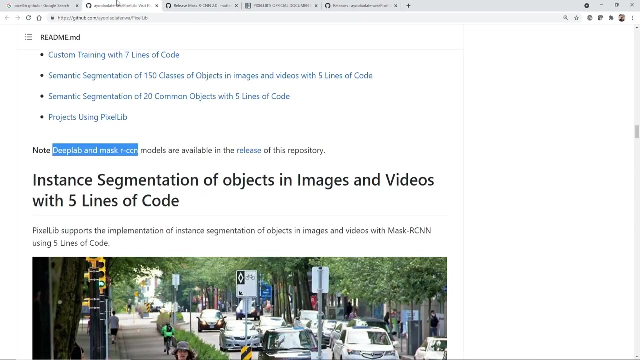 what all different, different types of models are there. One is deep lab and one is masked RCNN, which they have actually used. And remember, guys, the, the, the. you know the inference part is very, very quick. if you are also using this, So just go over here, Okay, And you can download this mask RCNN, Coco dot h5. Right, So this RCNN is basically trained on the Coco dataset, So what you have to do, go over here. there is have. there is something called a tutorial on back background editing in. 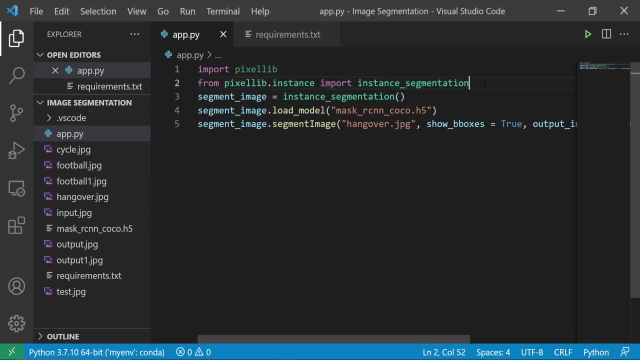 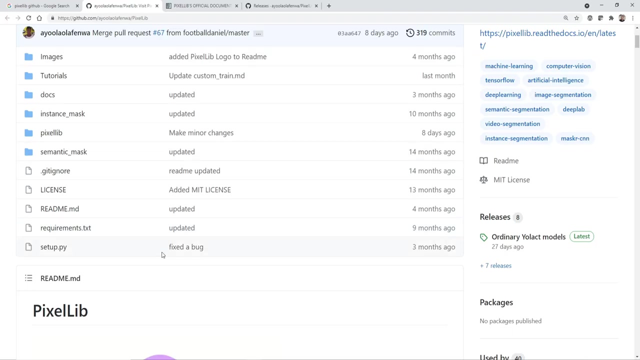 instance segmentation. So fine, guys, we have actually imported both this library and we are going to use this instance segmentation for doing the segmentation, And for this we also required a library, probably like our CNN, and also that it will be able to do the object detection And, based on that, it will also be able to show the boxes to us, right? So for that we are going to use this h5 file. And where did I get this h55?? Because it is already given away. if I go down, you'll be able to see all the examples over here, And they have released. 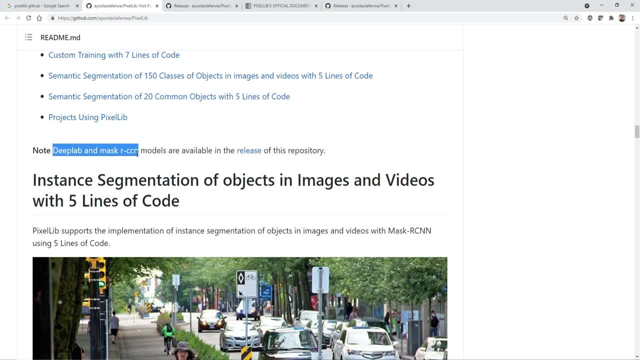 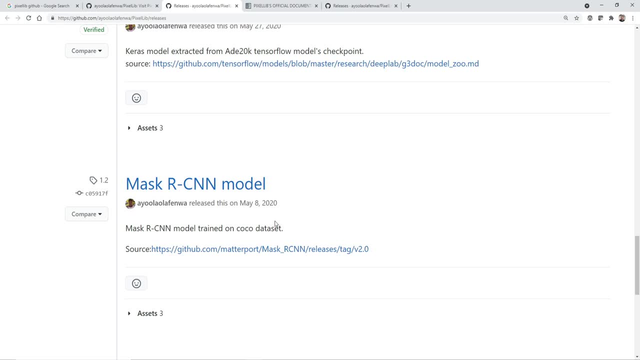 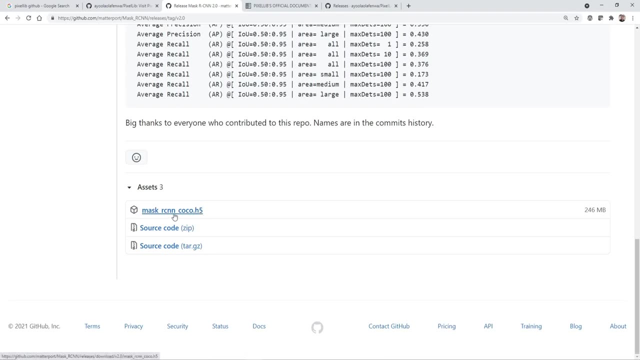 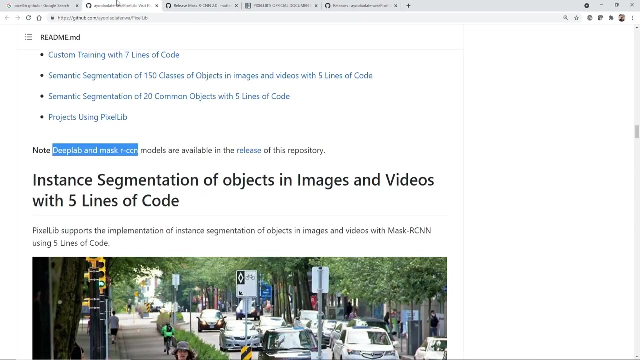 what all different, different types of models are there. One is deep lab and one is masked RCNN, which they have actually used. And remember, guys, the, the, the. you know the inference part is very, very quick. if you are also using this, So just go over here, Okay, And you can download this mask RCNN, Coco dot h5. Right, So this RCNN is basically trained on the Coco dataset, So what you have to do, go over here. there is have. there is something called a tutorial on back background editing in. 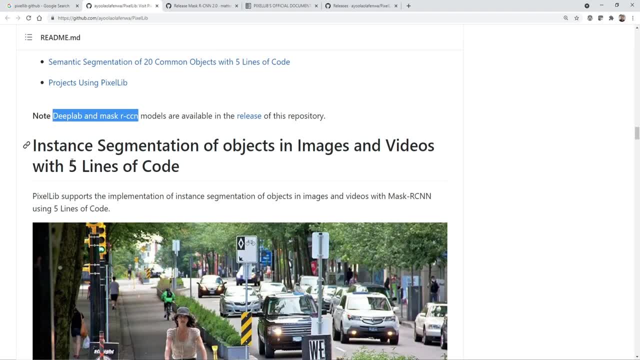 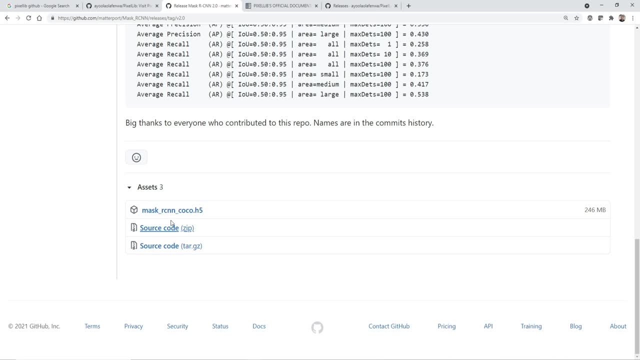 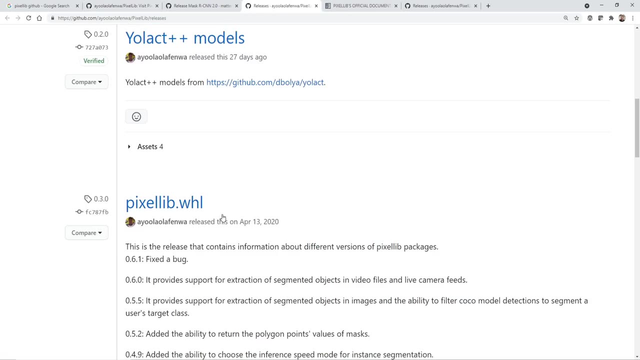 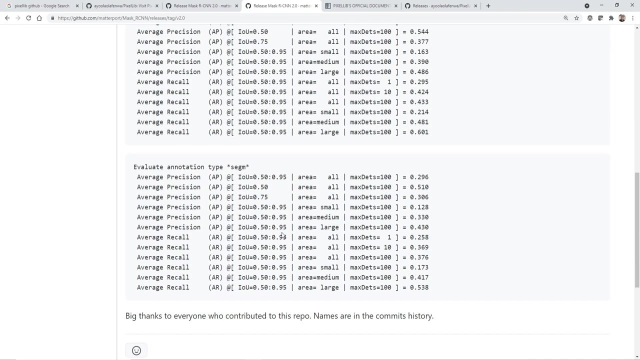 videos, And here you can actually see the. the note is there which says deep lab and mask RCNN are available in the release of this repository. So once you click this, you'll be able to go over here and you'll be able to select this. Okay, So again, let me just go and click it So you'll be getting this page and then go down, right the go down and just click this. Okay, So masked RCNN, And for this particular purpose we are going to use masked RCNN. Okay, Now, after we use this, after I download it- if I click this I'll get downloaded, And here you can. 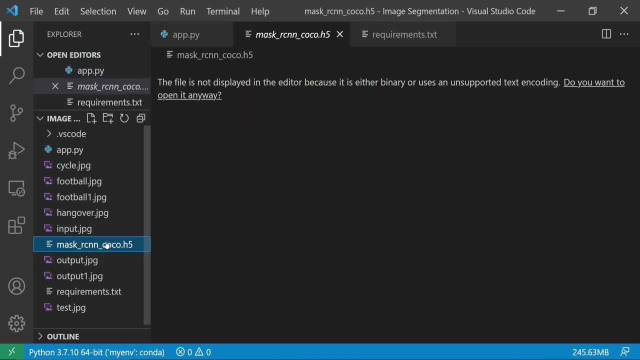 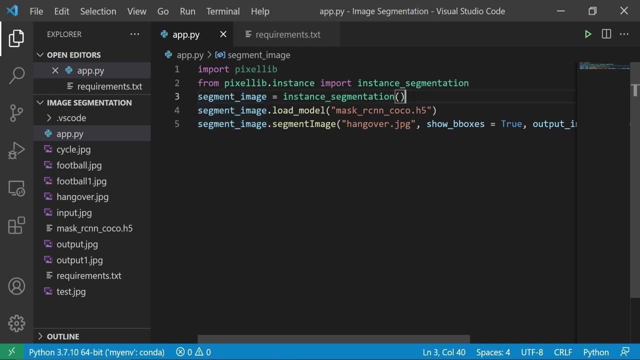 see that I'll be able to find this h5 file. So I've actually uploaded this in my same working location. Perfect, Then what I'm going to do? I'm going to use this segment image. First of all, we are going to initialize, with the help of instance segmentation, this will be an object, And then we are going to load this particular h5 file for the object detection purpose And along with that, we'll try to also do the segment image. So this is both object detection and image segmentation. Okay, So here in the segment image, the first image is basically your input image. 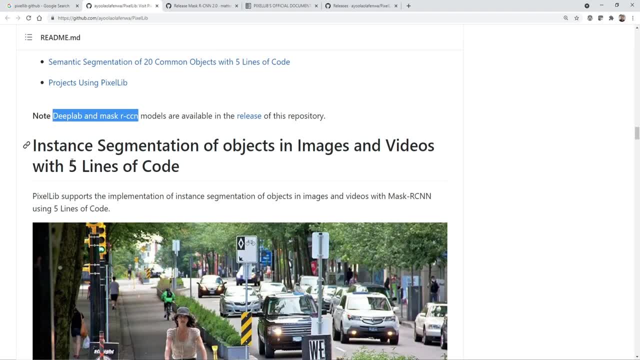 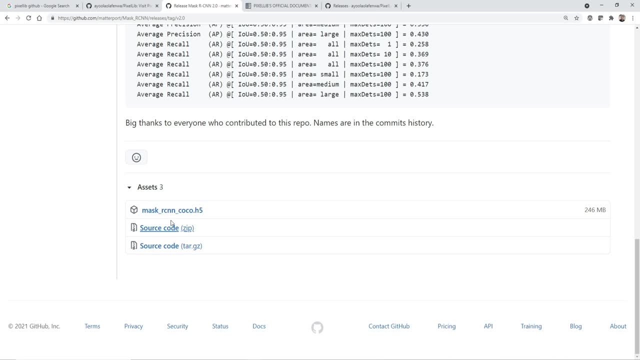 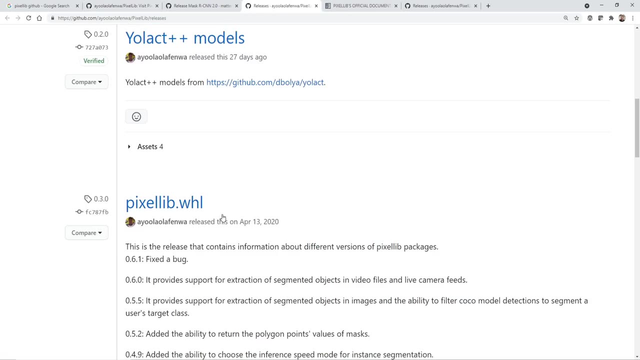 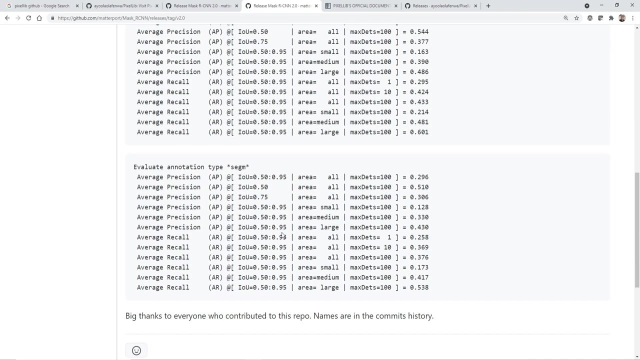 videos, And here you can actually see the. the note is there which says deep lab and mask RCNN are available in the release of this repository. So once you click this, you'll be able to go over here and you'll be able to select this. Okay, So again, let me just go and click it So you'll be getting this page and then go down, right the go down and just click this. Okay, So masked RCNN, And for this particular purpose we are going to use masked RCNN. Okay, Now, after we use this, after I download it- if I click this I'll get downloaded, And here you can. 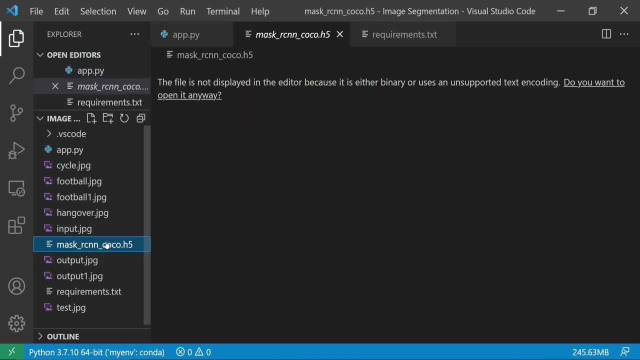 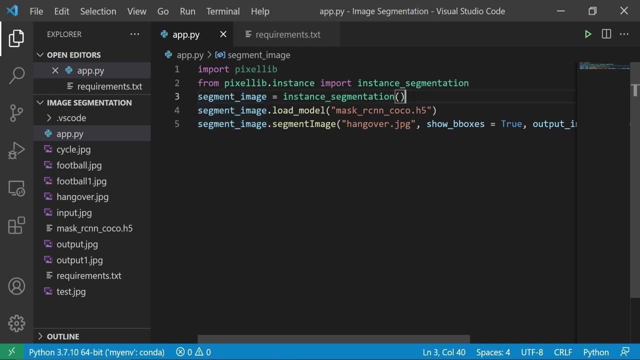 see that I'll be able to find this h5 file. So I've actually uploaded this in my same working location. Perfect, Then what I'm going to do? I'm going to use this segment image. First of all, we are going to initialize, with the help of instance segmentation, this will be an object, And then we are going to load this particular h5 file for the object detection purpose And along with that, we'll try to also do the segment image. So this is both object detection and image segmentation. Okay, So here in the segment image, the first image is basically your input image. 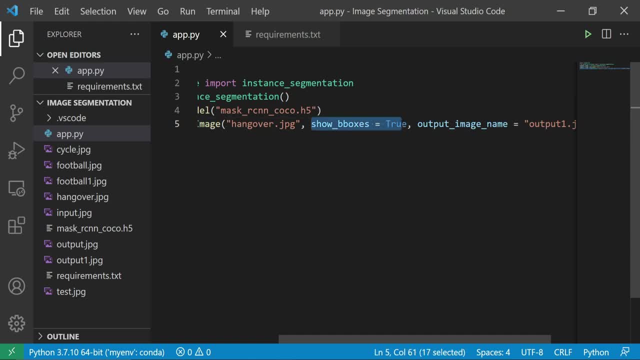 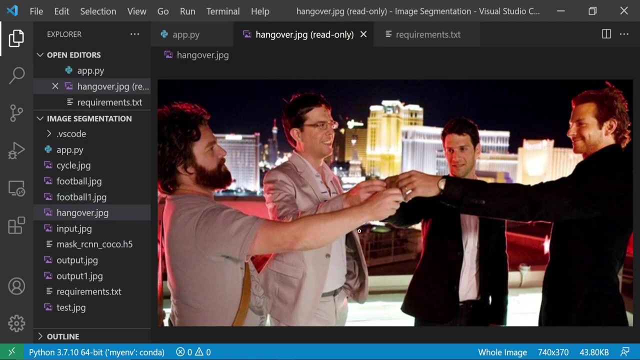 And then there will be a parameter which is called a show BB B boxes- is equal to true. you have to set it as true, Otherwise you'll be able to not be able to see the boxes. And after taking this image, after performing the image segmentation and object detection, you will be able to get the output name something like this: Right? So let's quickly run. right now I'm giving hangoverjpg. I hope everybody has seen the hangover image, right? So this particular movie, hangover, part one, I hope many people have seen it. So let's see how. 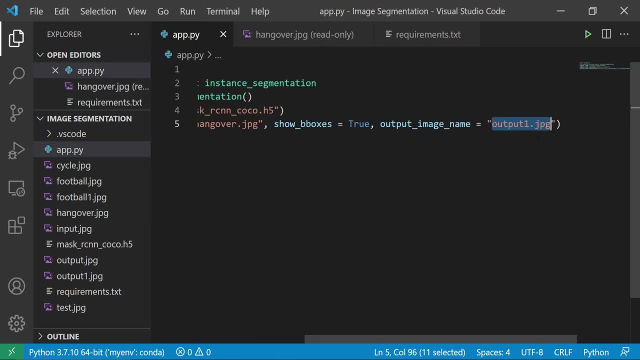 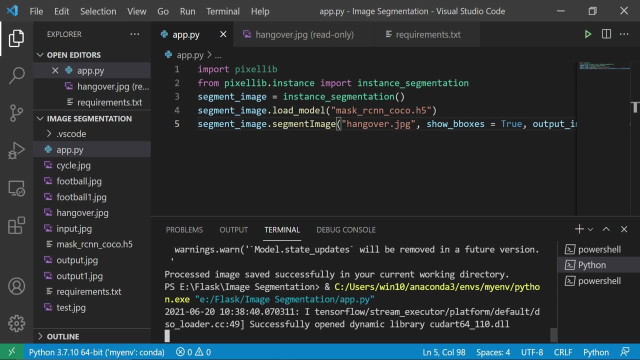 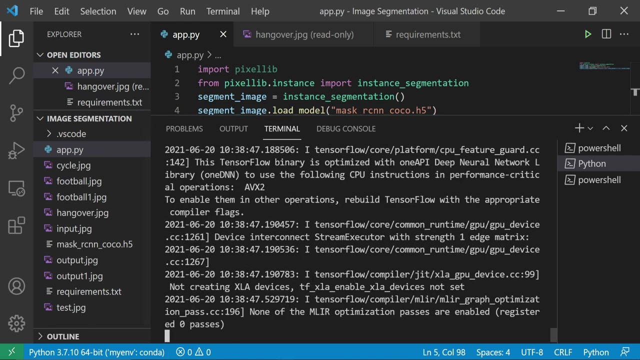 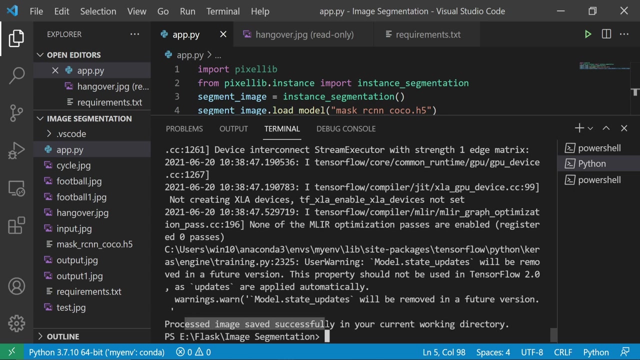 we are going to get an output. Once, then, output is basically created, you'll be able to get output one dot jpg. Okay, so let's go and run it. And here we go And make sure that you have all the libraries installed perfectly, guys. then only things will work. Okay, So I'm now executing this. you'll be able to see all the image. segmentation will be done and it will actually create an image called as output one. So here you can see processed image save successfully in the current working directory. And this is my output one. And if I want to show you the 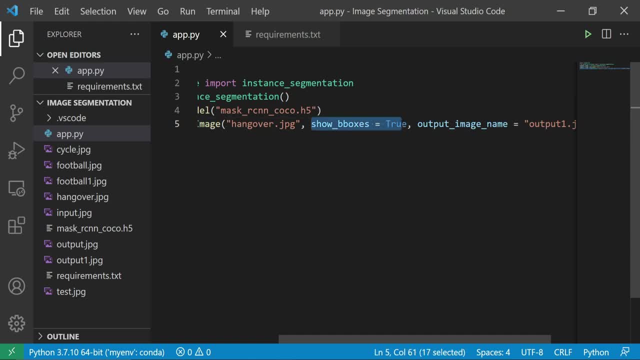 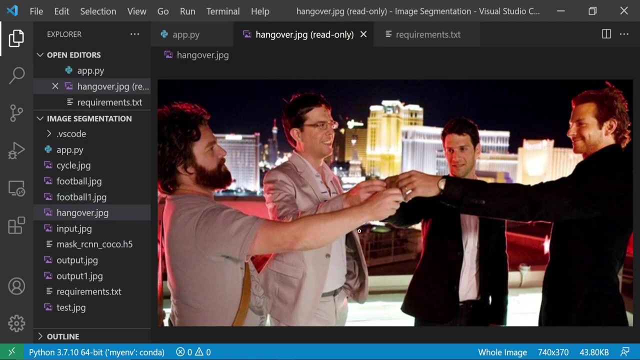 And then there will be a parameter which is called a show BB B boxes- is equal to true. you have to set it as true, Otherwise you'll be able to not be able to see the boxes. And after taking this image, after performing the image segmentation and object detection, you will be able to get the output name something like this: Right? So let's quickly run. right now I'm giving hangoverjpg. I hope everybody has seen the hangover image, right? So this particular movie, hangover, part one, I hope many people have seen it. So let's see how. 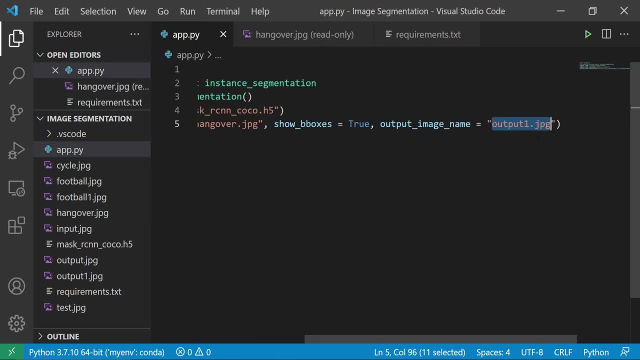 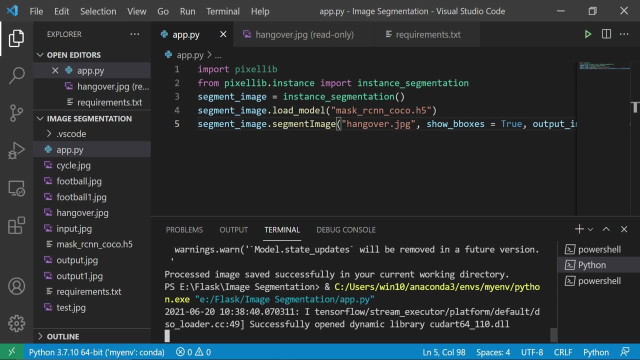 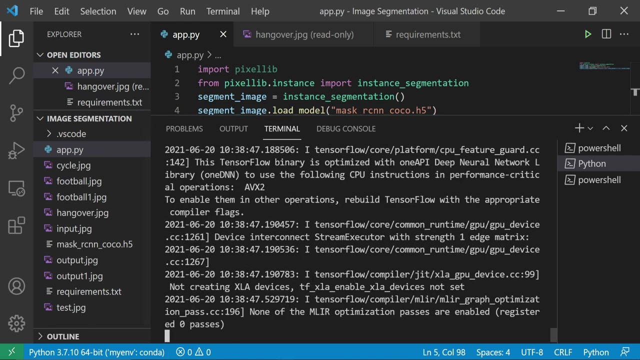 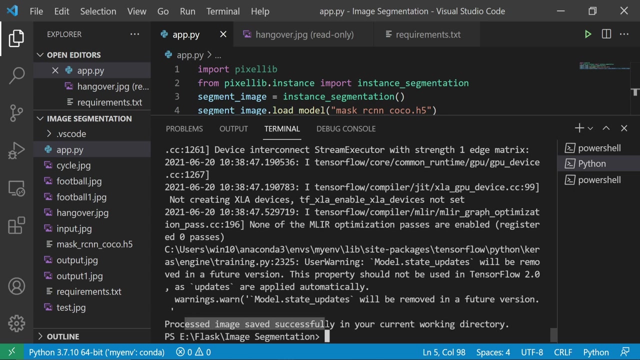 we are going to get an output. Once, then, output is basically created, you'll be able to get output one dot jpg. Okay, so let's go and run it. And here we go And make sure that you have all the libraries installed perfectly, guys. then only things will work. Okay, So I'm now executing this. you'll be able to see all the image. segmentation will be done and it will actually create an image called as output one. So here you can see processed image save successfully in the current working directory. And this is my output one. And if I want to show you the 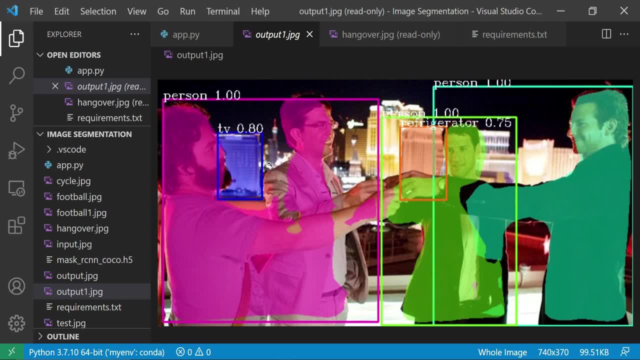 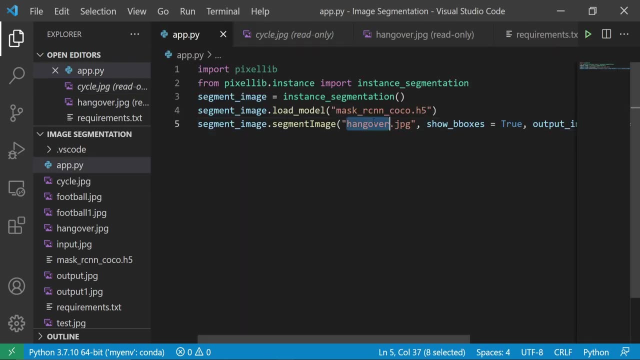 image. this is how it looks like. Yes, it is detecting this building as TV, but person is detected, person is defected and refrigerator because this looks like a refrigerator itself. But amazing accuracy. Let's try some other one. So here I'm going to give you this image: Okay, cycle dot jpg, Let's see. So I'm just going to try this one cycle dot jpg And probably give my image as output dot, or I'll say: output two dot jpg. Okay, And probably I'll run it. 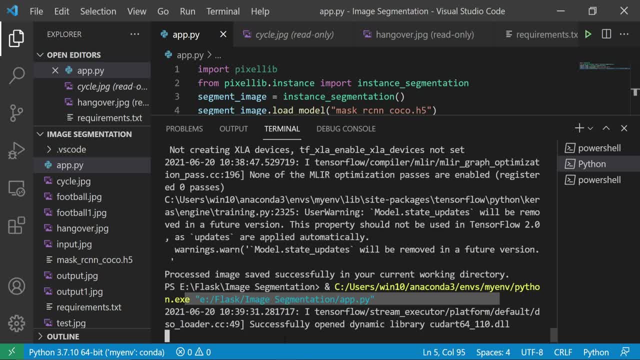 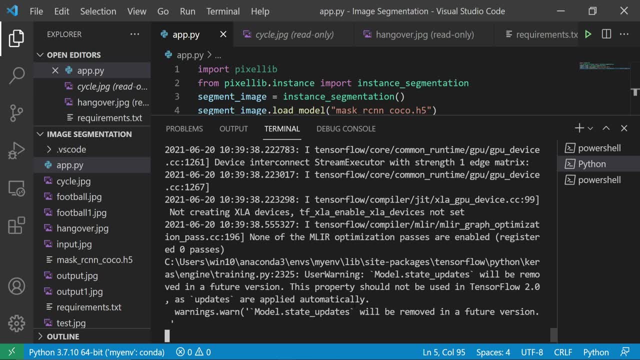 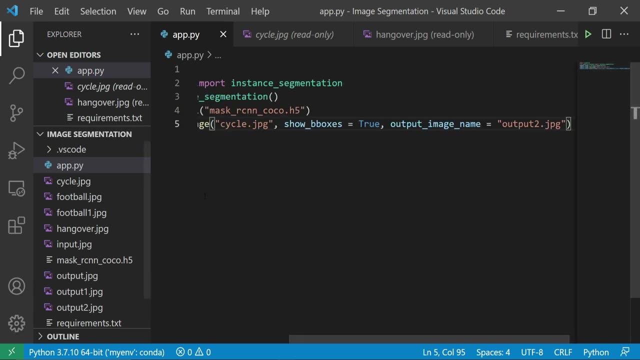 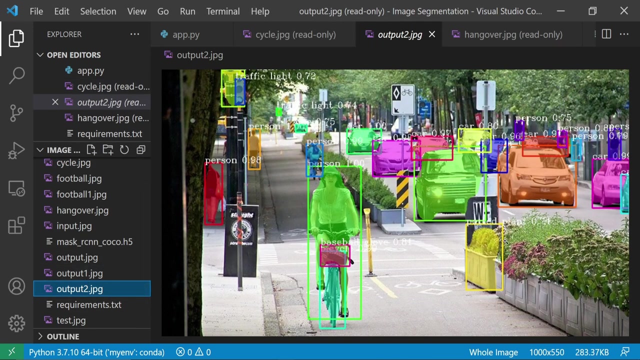 So probably this will also take some time to run it And again, it depends on your system, also based on the inferences that you're actually getting. Okay, So quickly, quickly, let's, let's see: Yes, it is saved. What is my file name? output two. So initially I had this specific image And now I'm able to get this specific image And you can see how accurately everything is there. You can see this petted plant, you can see person, cars, this, this, everything. 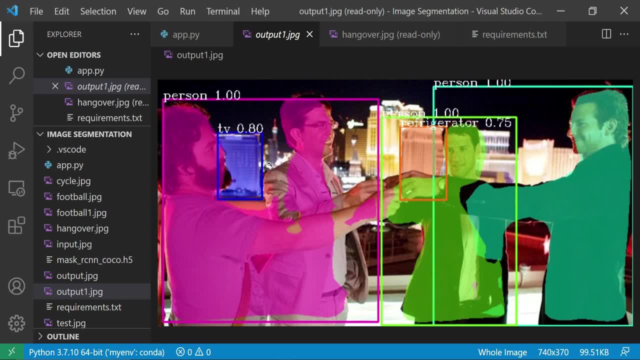 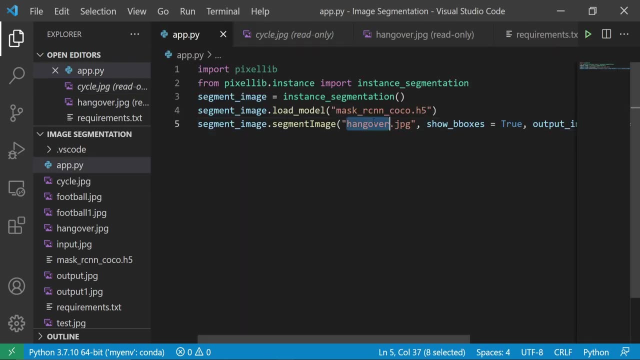 image. this is how it looks like. Yes, it is detecting this building as TV, but person is detected, person is defected and refrigerator because this looks like a refrigerator itself. But amazing accuracy. Let's try some other one. So here I'm going to give you this image: Okay, cycle dot jpg, Let's see. So I'm just going to try this one cycle dot jpg And probably give my image as output dot, or I'll say: output two dot jpg. Okay, And probably I'll run it. 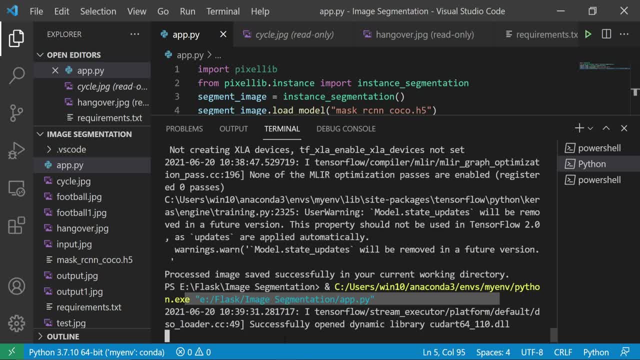 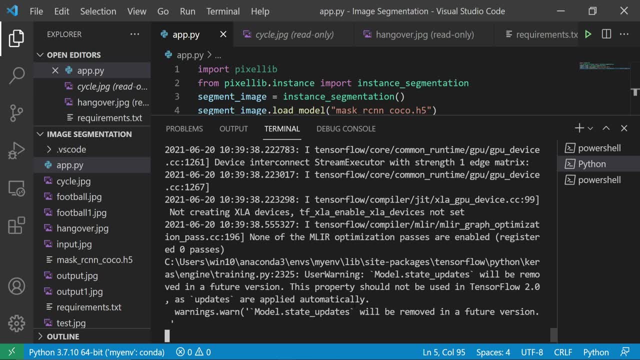 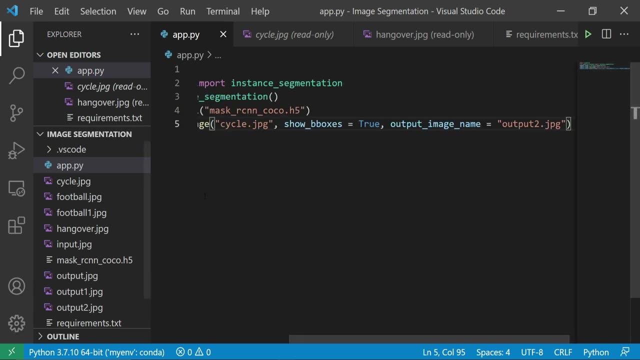 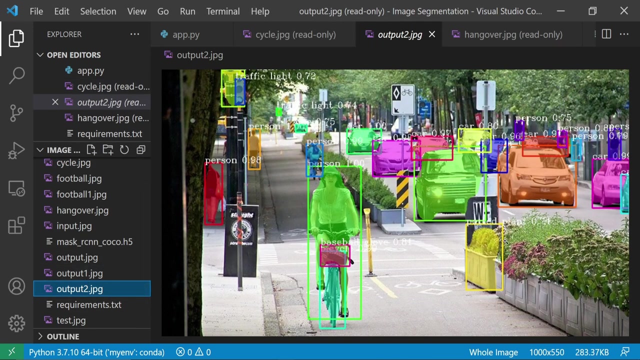 So probably this will also take some time to run it And again, it depends on your system, also based on the inferences that you're actually getting. Okay, So quickly, quickly, let's, let's see: Yes, it is saved. What is my file name? output two. So initially I had this specific image And now I'm able to get this specific image And you can see how accurately everything is there. You can see this petted plant, you can see person, cars, this, this, everything. 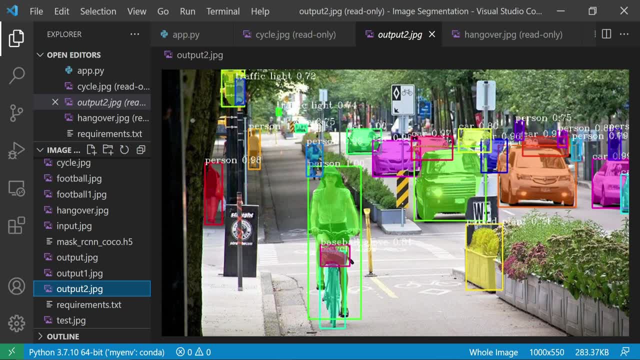 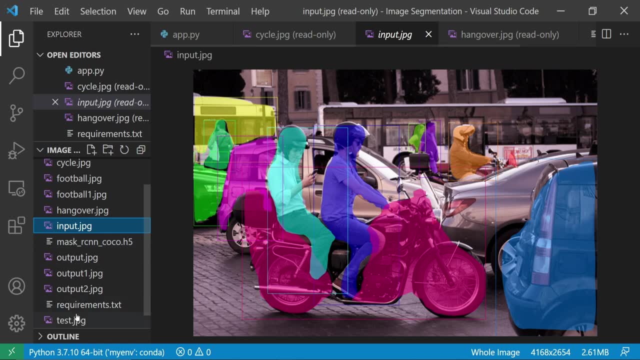 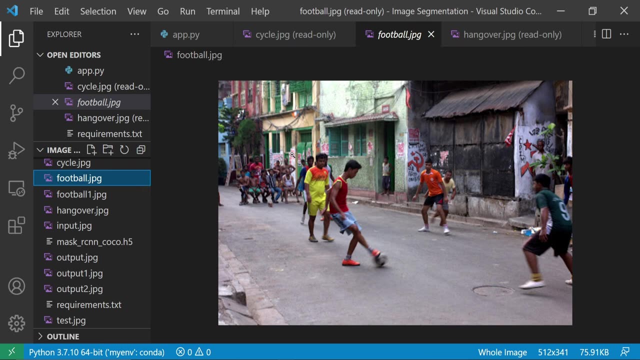 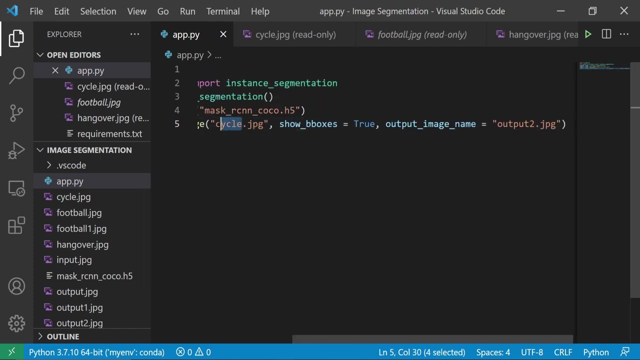 Everything is there, Amazingly right. It is being able to. even traffic light is given over here, Right. So this is my second example. Third example: I can also take something like this: This is my test dot jpg. you'll be able to see input dot jpg over here. Let's see this one: football. I can see that it is not that clear, But let me try this one also. So here I can say football dot jpg, Okay, football dot jpg. And here I'm just going to say output two. 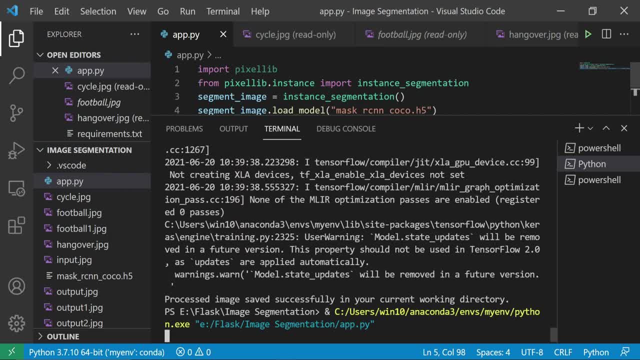 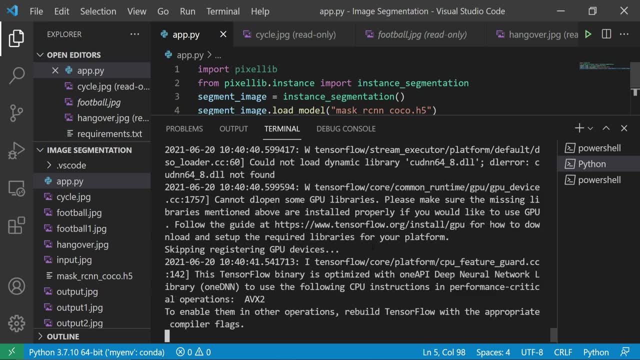 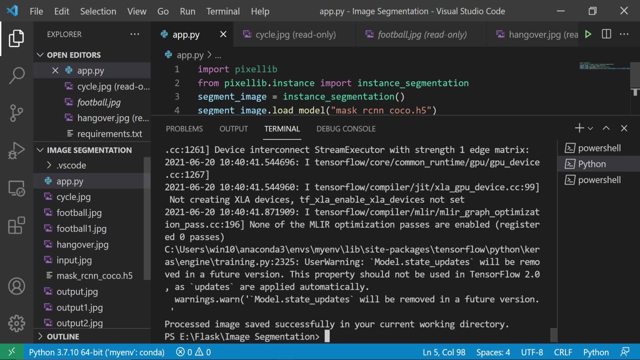 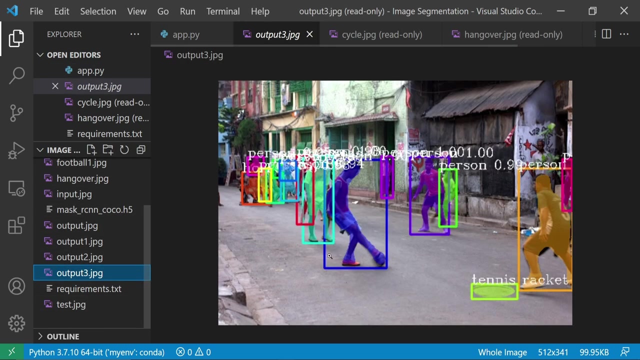 Three: So just with this three line of code and in the upcoming videos I'll also showing you how to do this. in videos, Okay, it will be pretty much amazing. in live streams Also, I'll be able to show you how these things work because I've been exploring, with respect to image segmentation, Trust me, the older approach that we used to do. And you may be thinking, Chris, how to do custom training. don't worry about that, That also. I'll try to show custom training of different images and all also you can actually do. So this is my output. three. Now here you can see that, yes, within this also it is being properly determined person and all. 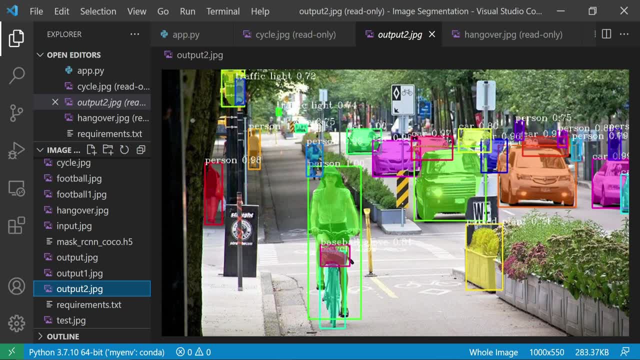 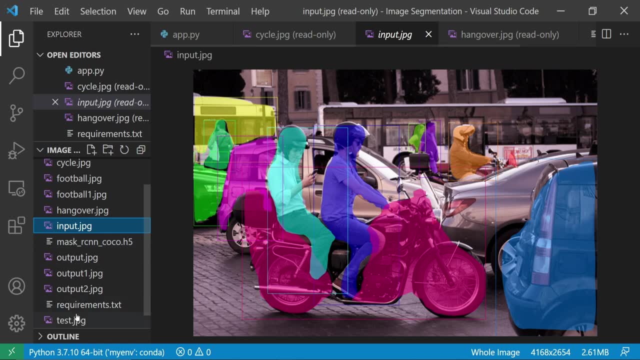 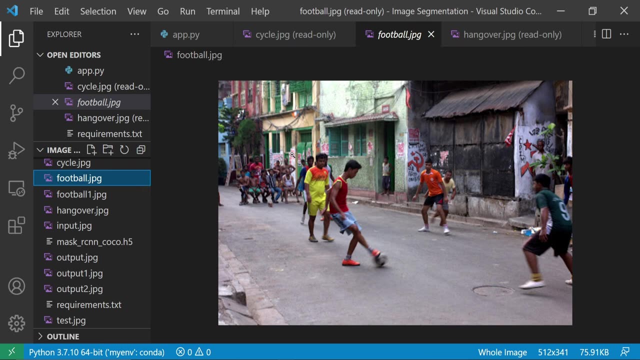 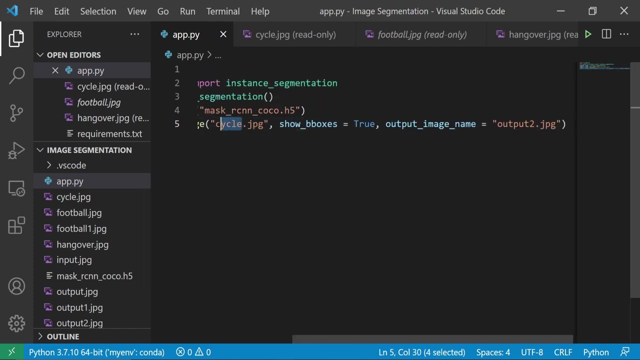 Everything is there, Amazingly right. It is being able to. even traffic light is given over here, Right. So this is my second example. Third example: I can also take something like this: This is my test dot jpg. you'll be able to see input dot jpg over here. Let's see this one: football. I can see that it is not that clear, But let me try this one also. So here I can say football dot jpg, Okay, football dot jpg. And here I'm just going to say output two. 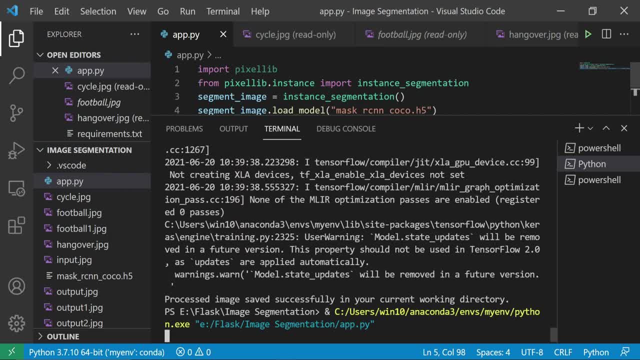 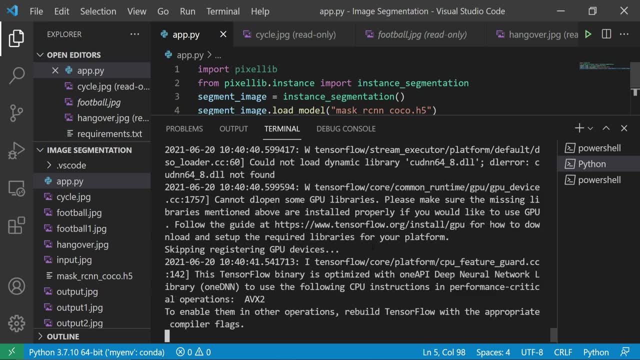 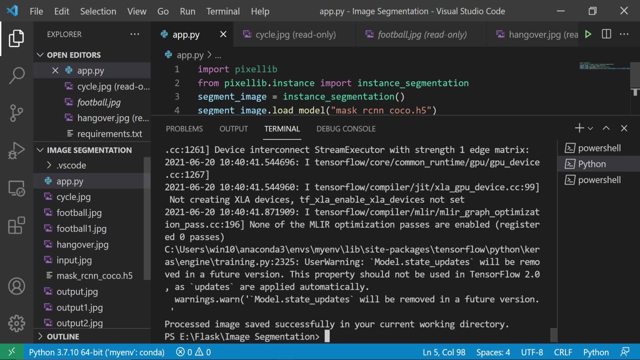 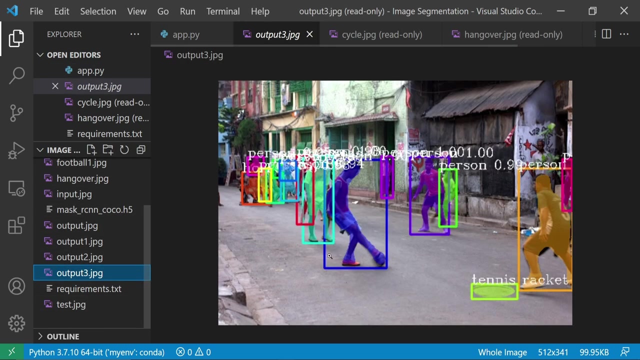 Three: So just with this three line of code and in the upcoming videos I'll also showing you how to do this. in videos, Okay, it will be pretty much amazing. in live streams Also, I'll be able to show you how these things work because I've been exploring, with respect to image segmentation, Trust me, the older approach that we used to do. And you may be thinking, Chris, how to do custom training. don't worry about that, That also. I'll try to show custom training of different images and all also you can actually do. So this is my output. three. Now here you can see that, yes, within this also it is being properly determined person and all. 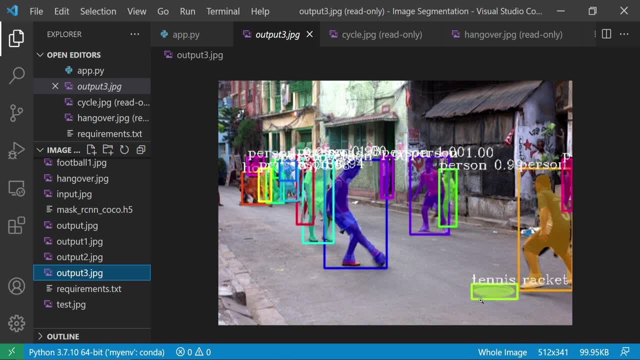 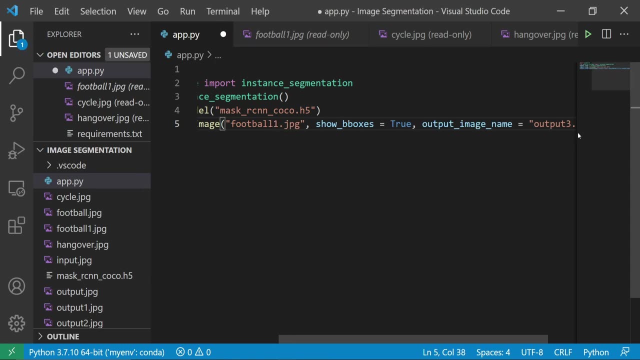 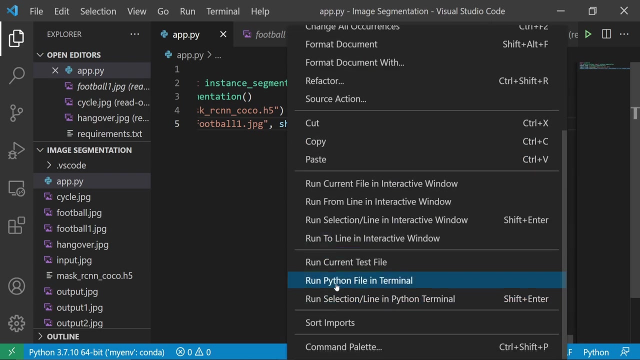 But here you can see, the tennis is basically determined. This was not tennis actually. Yes, some, some amount of error is there. Definitely not 100% accuracy, but, yes, a good accuracy, altogether Right, Let's see one more. So I have this football one dot jpg. Let's see this also, if I'm able to get in a proper way And I have output four, Perfect, And let me run it. 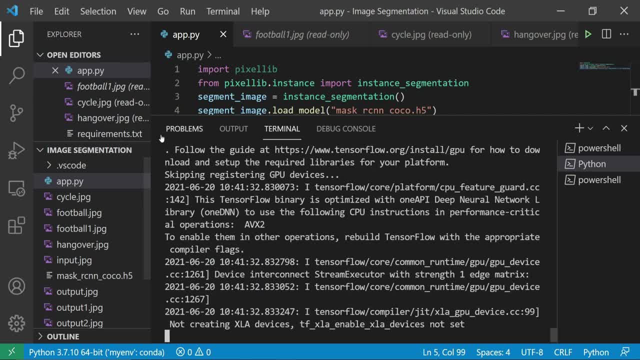 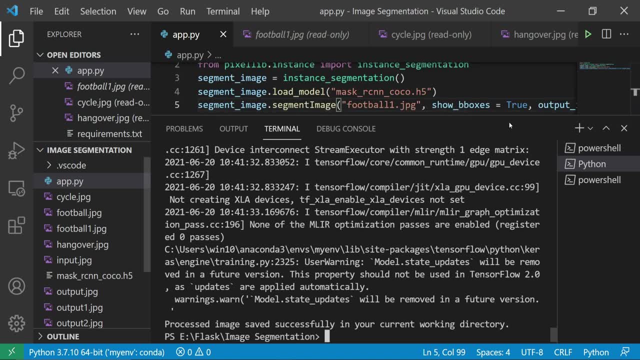 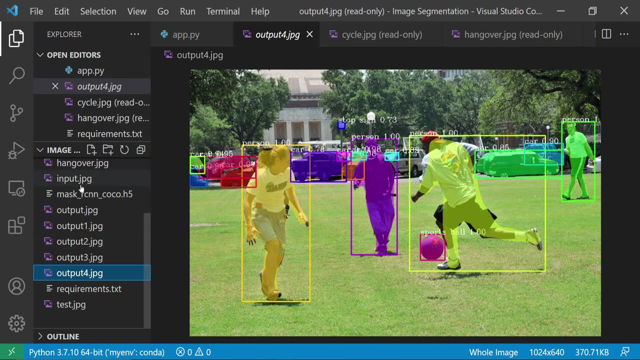 So here you'll be able to see. now I think it will work perfectly fine And I'm just giving my input and output image by just using this RCNN model And I think it will work. So it is good saved. Now let me see my output four. So here you can see that this was my initial image. Sorry, this was my initial image. Now, after doing the segmentation and all, I'm actually getting something like this, And here clearly everything is basically getting determined, even stop sign also. So I hope you like this particular video. Please do subscribe to the channel. 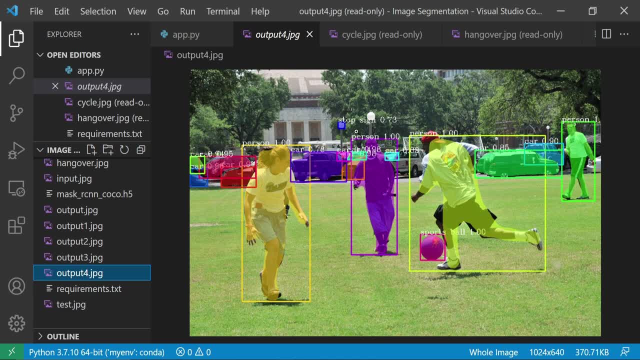 If you're not already subscribed, and I'll put all this particular thing in my GitHub so that you can actually work it out Right. I'll see you in the next video. Have a great day. Thank you, one doll, Bye, bye.